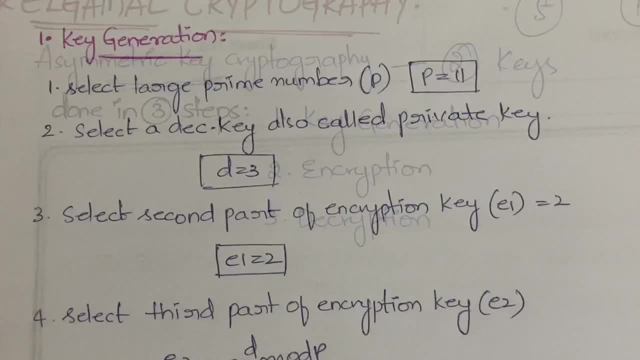 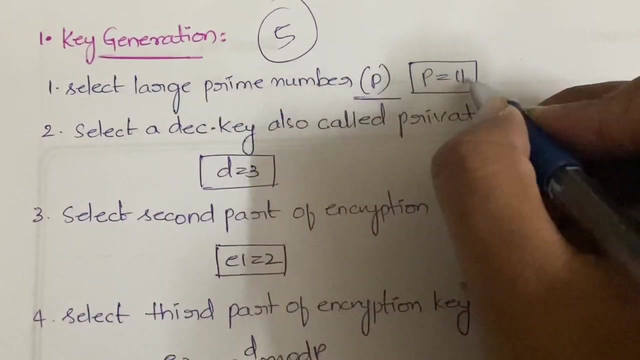 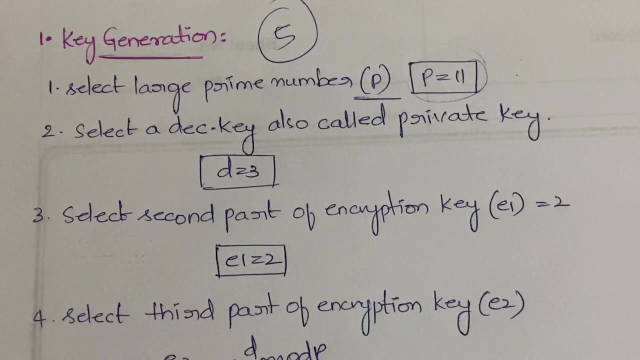 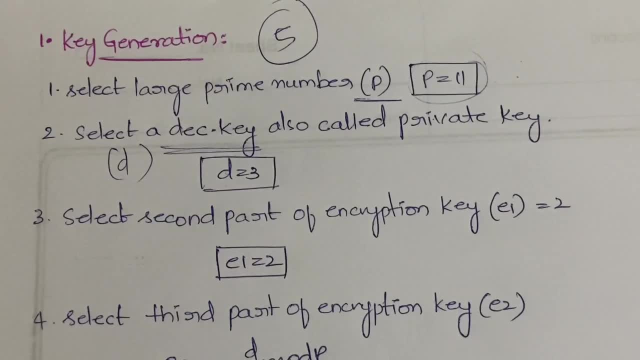 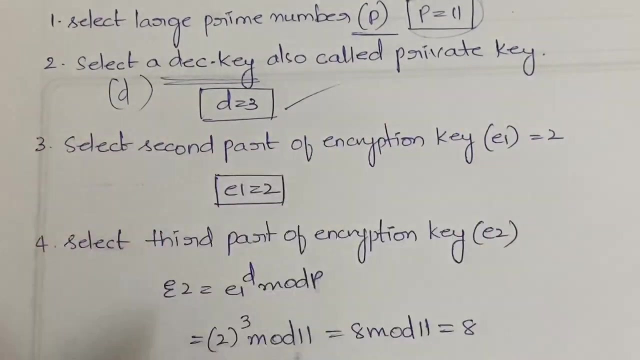 need to select the decryption key, which is denoted by D And it is also called as the private key. Got it. So you have to select a private key. Private key also, you have to select it on your own itself. Got it Now. once you select your private key- So we have selected, D is equal to 3.. Done. In the third step, what you have to do is you have both second part and third part of the encryption key here. Okay, So second part. 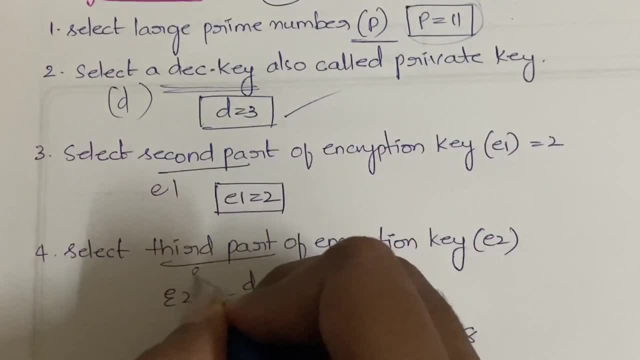 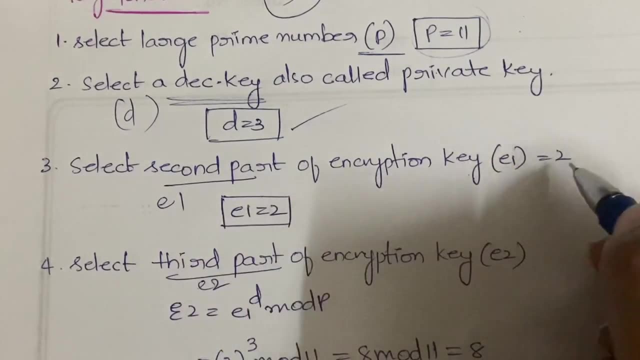 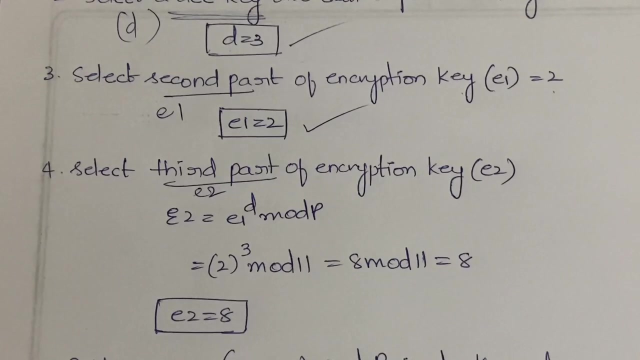 of encryption key is denoted with e1. third part of encryption key is denoted with e2. okay, so you need to first select the second part of encryption, which is e1, and we have selected it as e2, sorry, 2. okay, so e1 is equal to 2 done in the fourth step. what you have to do is you need to calculate the. 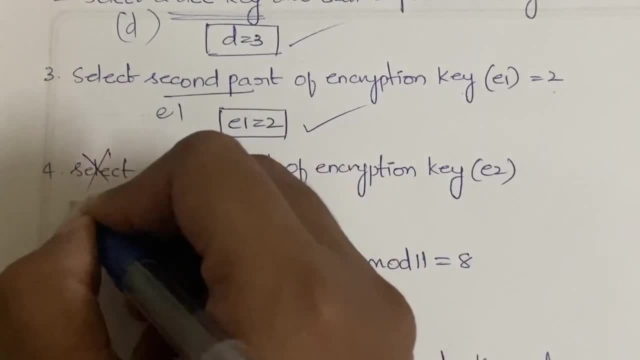 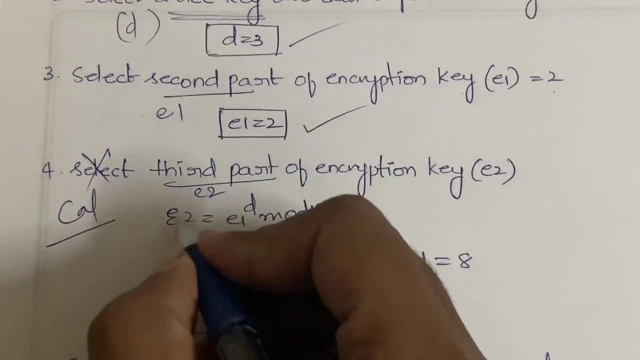 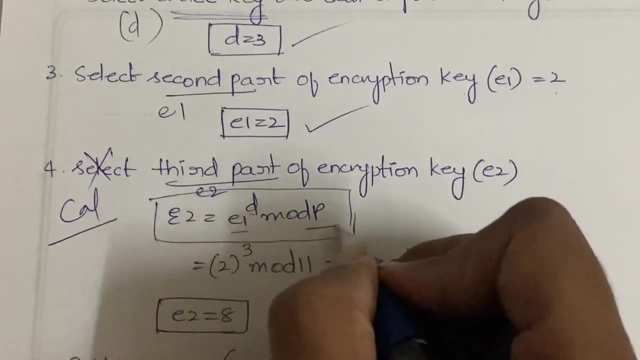 third part of the encryption key. so here, instead of select, you can use the word calculate, because you are using- you are not assuming it right- you are calculating with the existing value. so that will be equal to e2, will be equal to e1. power d mod p. we have e1, we have d and we have p, right. 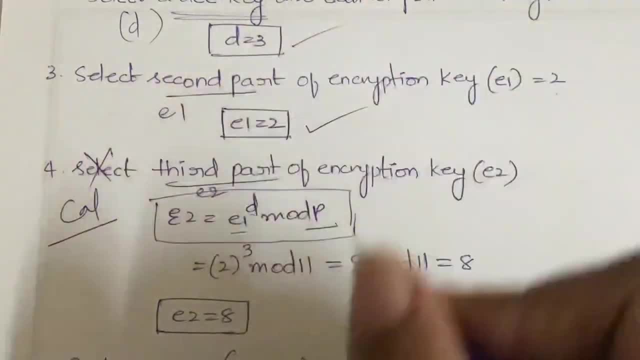 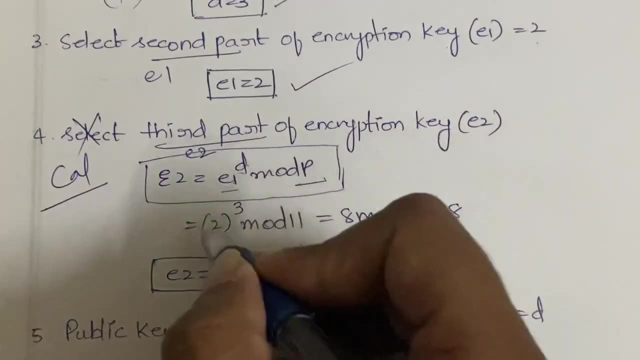 so e1 is nothing but 2 and d is nothing but 3 and p is nothing. but here we have assumed a prime number which is 11. okay, so the which will be equal to 2 power 3 mod 11, which is 8 mod 11. again, it. 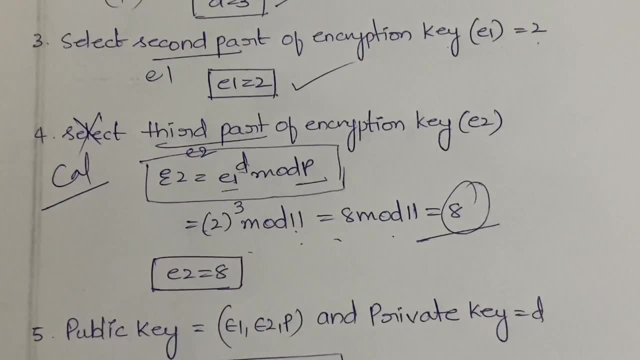 results in 8 itself got it. we got the value of e2 as well. we now have the values of p, d, e1, e2, 2. right now. in the next step, what you do is you will be calculating the public key. so how do you? 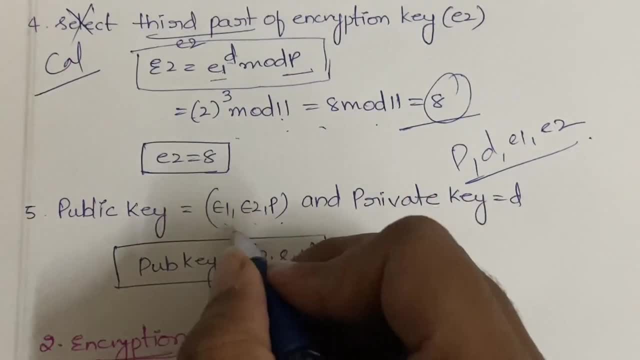 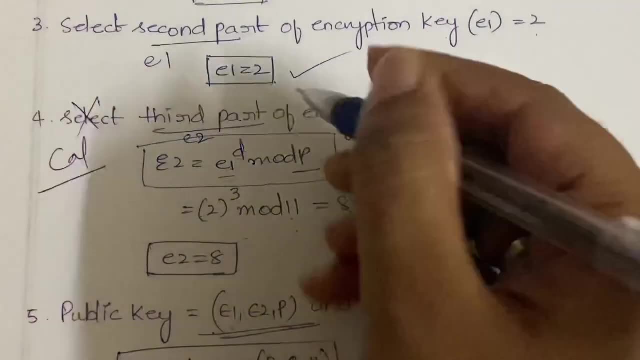 get the public key, e 1 comma e, 2 comma p. so this is the standard form for public key in this algorithm. so e 1 is what, e, 1 is 2, e 2 is 8 and p is 11. so 2 comma 8 comma, 11 is the public key and the private. 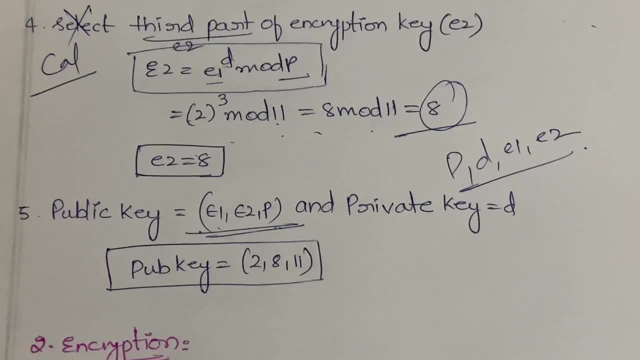 key is nothing but the decryption key, which we have already assumed, which is equal to 3. okay, done. now we have the public key and private key, so both the keys are generated. so the first step, key generation, is completed. since both keys are generated in the second step, what you're doing? 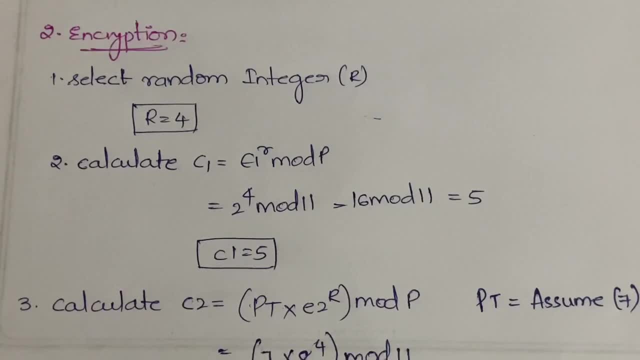 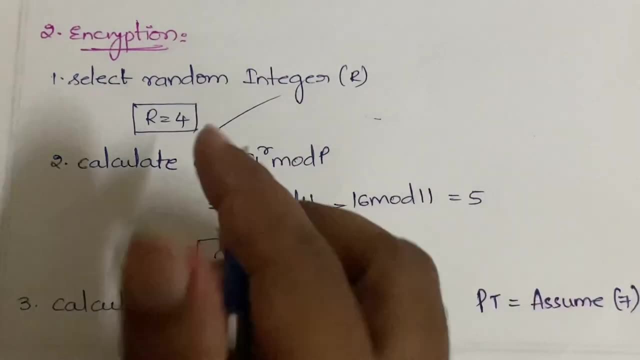 you're doing the encryption. so, in case of encryption, what you do is first you will be selecting some random integer, r. okay, so that we have selected it as r is equal to 4. done in the second step, what you do is you will be calculating the value of c1, c1 and c2 here represents the. 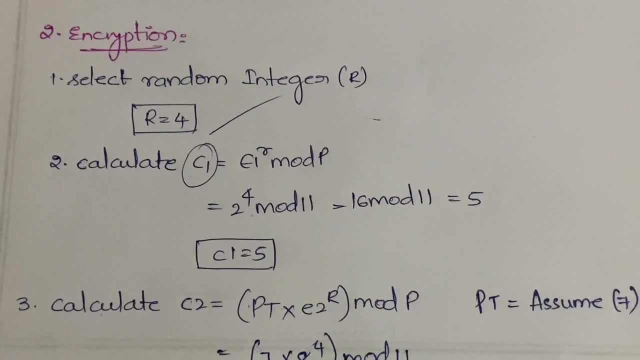 cipher text, got it. so here you are calculating c1 and c2. you will be calculating the value of c1, c1 and c2. here represents the cipher text, got it. so here c1 and c1 is equal to e1, power, r mod p. what is the value of e1, 2 and what r? we have assumed 4. 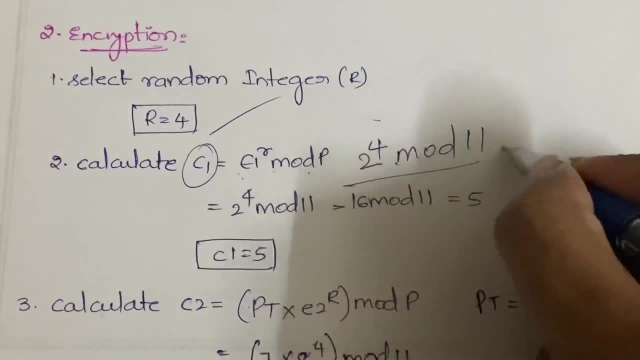 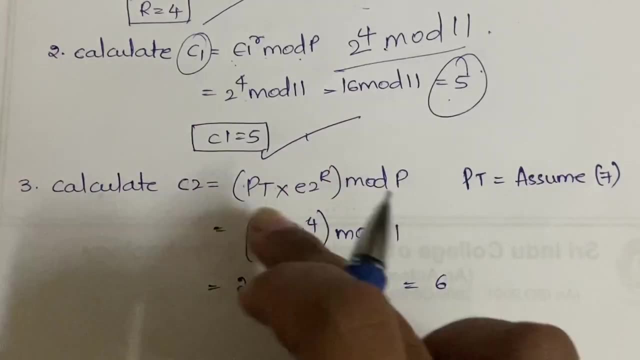 2 power 4 mod p is nothing but 11, so 16 mod 11, which will be equal to 5. so we got the value of c1 as 5 done. now you have to calculate the value of c2. how do you do it? pt into e2: power r mod p here. 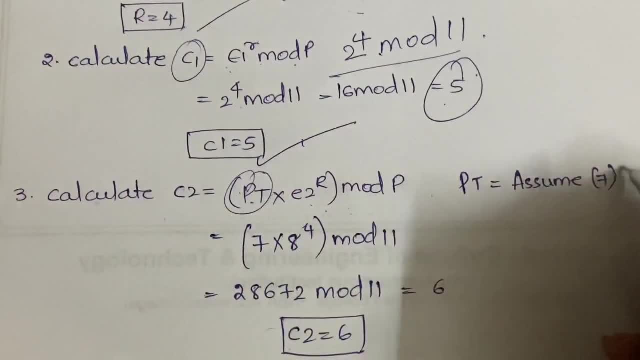 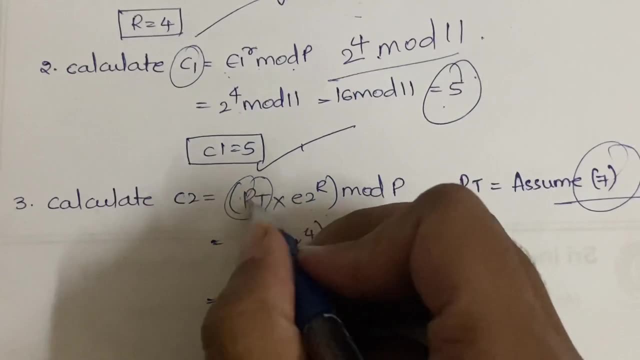 pt is nothing but the plain text. again, you will be assuming it and we have assumed it to be as 7. okay, now how do you calculate the c2? so So Pt is nothing but 7, we have assumed, and E2: we got it as 8.. 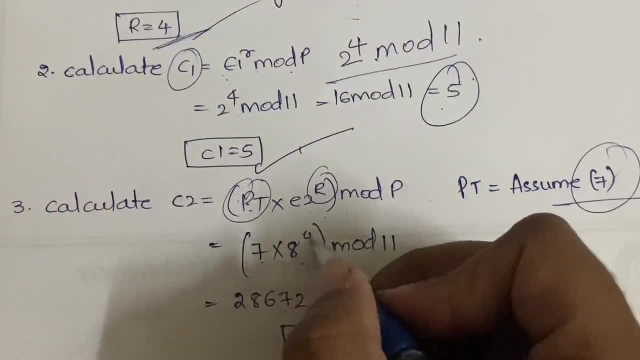 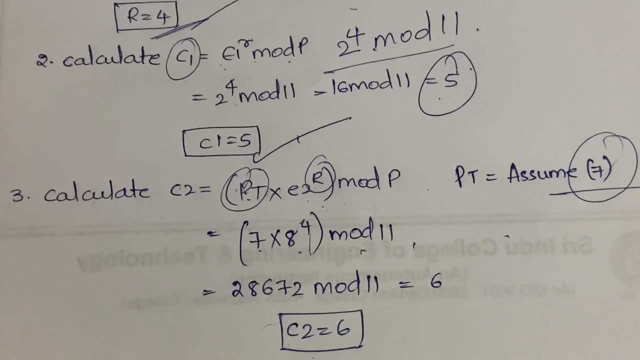 So 8 power R we have assumed as 4 here, power 4 mod 11.. So that you will be getting- you can do this in the calculator, However, since you are allowed to take the calc with you, So then you will be getting the value of C2 as 6, right. 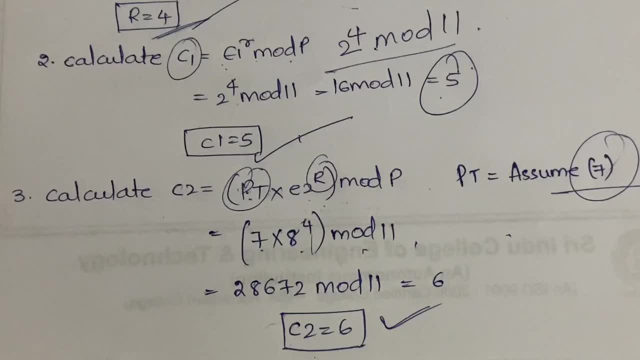 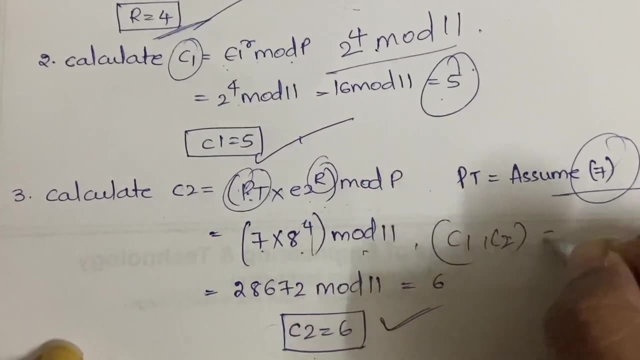 Now we are done with calculating C1 comma C2, right, This is nothing but the ciphertext. So what is C1 comma C2 now? So C1 comma C2 will be equal to 5 comma 6.. So we are done. we have obtained the ciphertext as well.